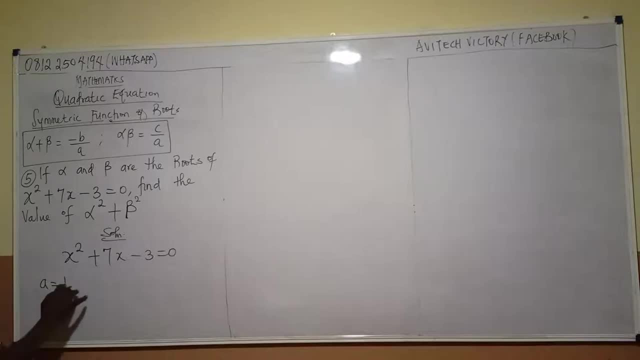 So you then bring out a, and a is worth 1.. Then bring out b- b is worth 7.. Then it all becomes c minus 3.. So a is 1, b is 7, c is worth minus 3.. So let us then proceed. Next, what we're going to do is: 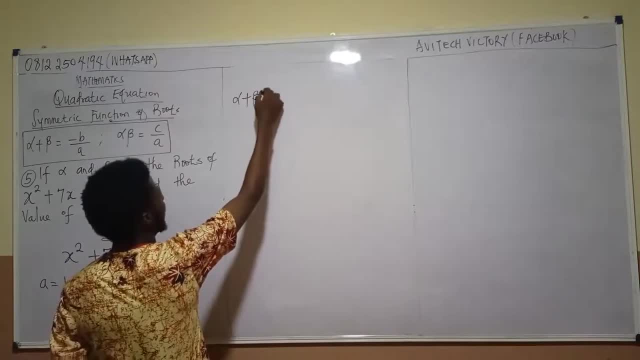 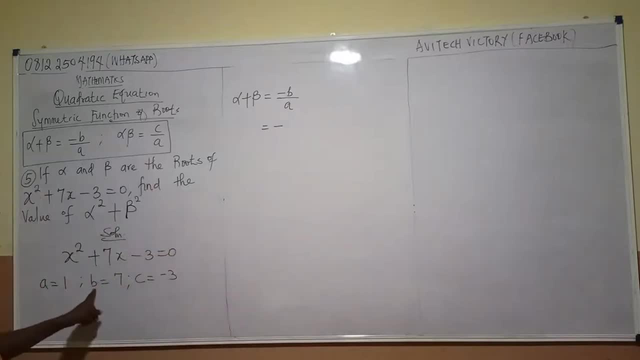 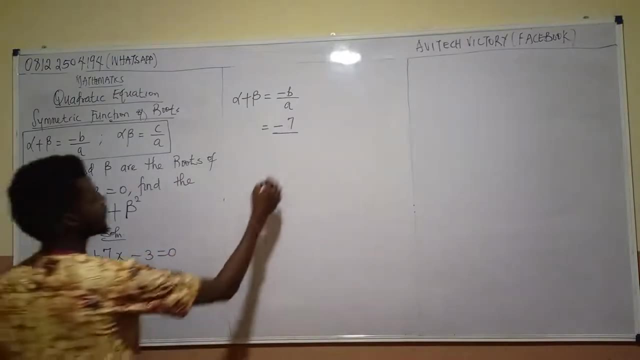 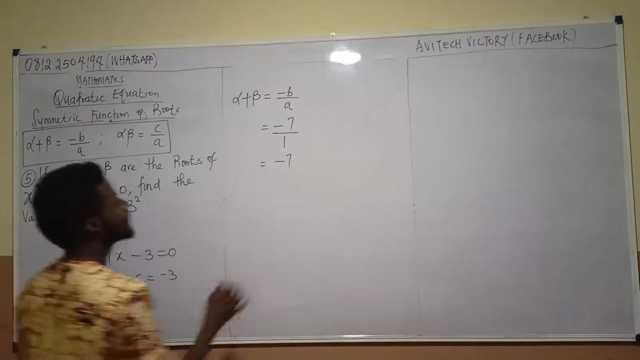 this is minus what is b in the question. b is what seven. so if b is seven divided by what will become? our a is one. so finally, minus seven divided by one is minus what seven. so that's alpha plus beta. what would then become alpha beta? alpha beta would then become: 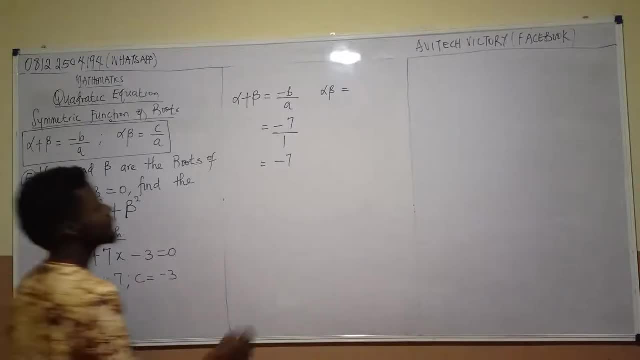 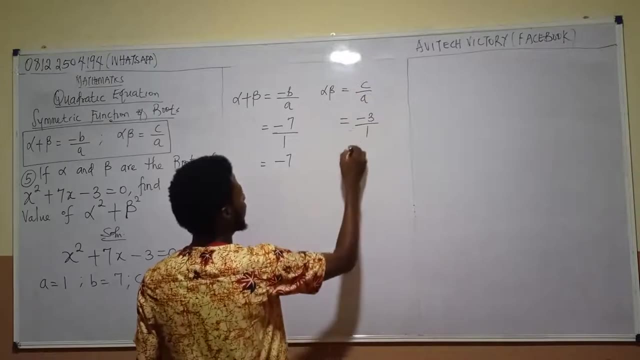 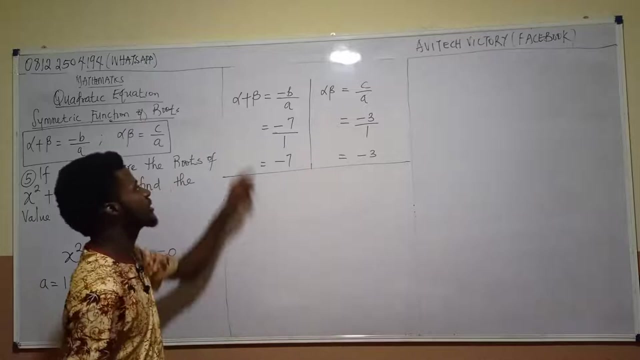 c over a, so that's c over a, and what is our c minus three over what is our a one? so i'll just give to you minus three. so that means alpha plus beta is minus seven, alpha beta is minus three. now look at this question very well. 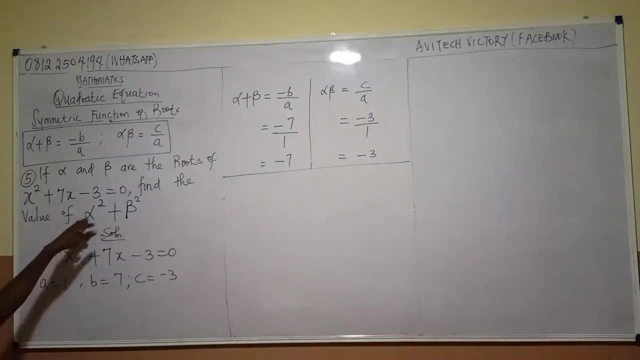 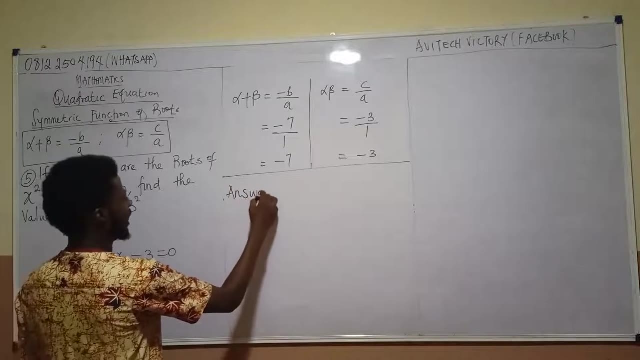 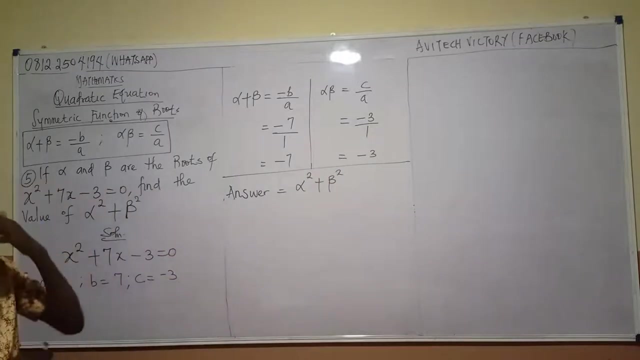 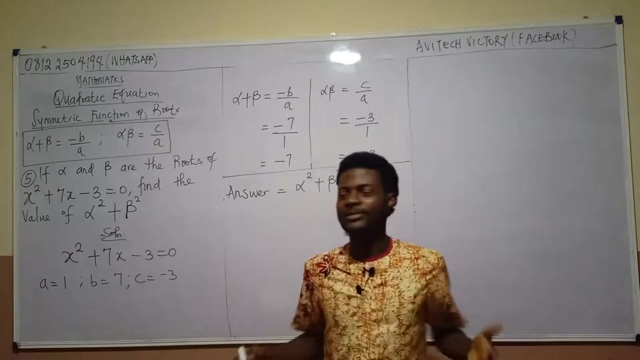 the question says: find the value of alpha squared plus beta squared. very sweet question. so the question says: you find the answer of alpha squared plus beta squared? wow really. should i give you some minutes to solve the question? should i give you some time to solve it? do you want to try? 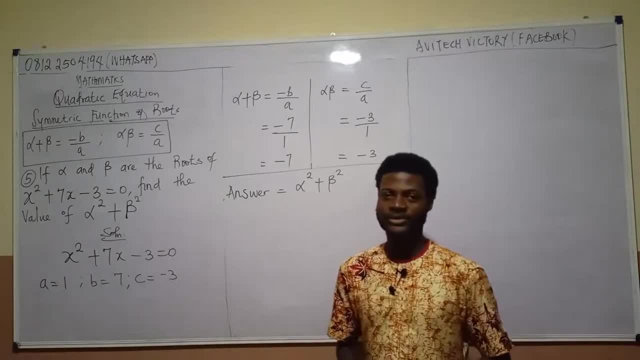 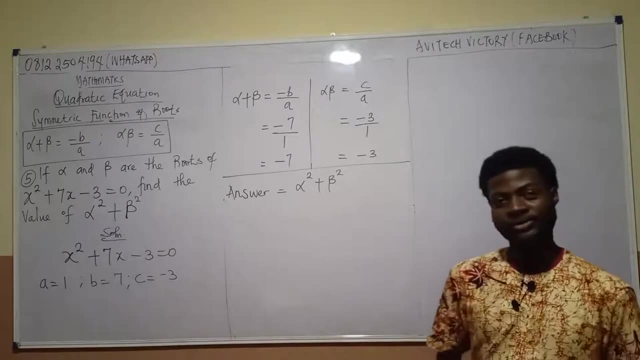 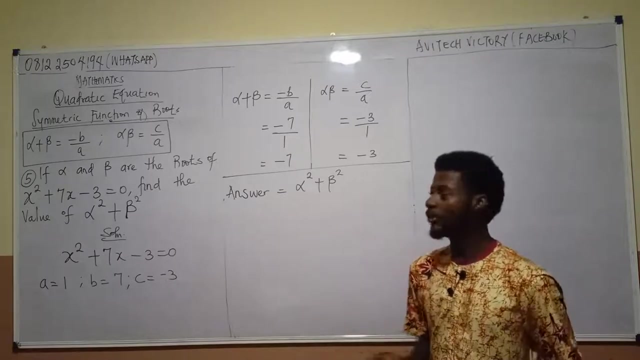 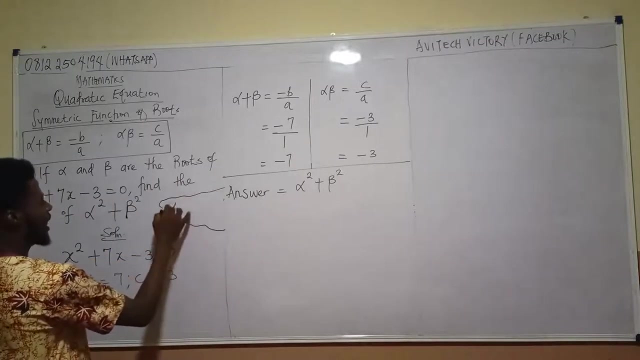 to solve it without moving forward. so let me give you some time to solve. please give to one what, okay? so let me give you three seconds. three, two, one. okay, now look at this, look at this, please, and please, please and please. it is not acceptable anywhere in this life that is not acceptable. that alpha squared. 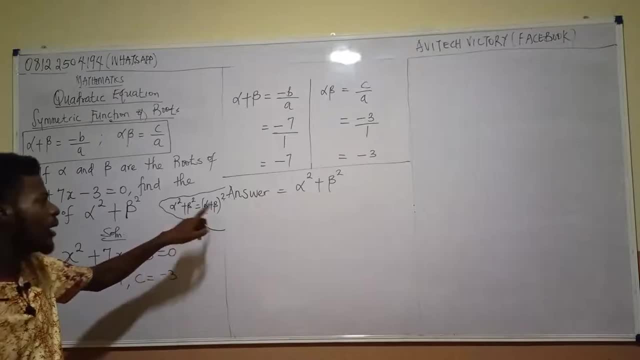 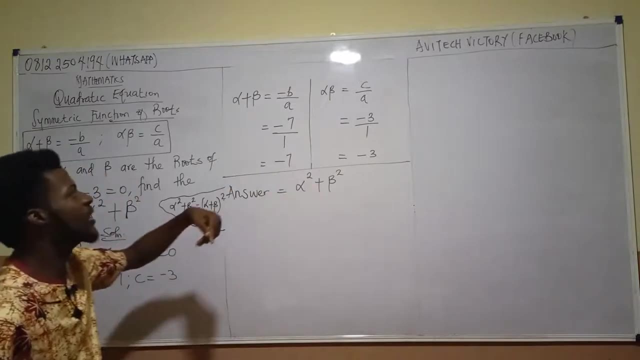 If you're trying to do this, you would be wrong, But let us try to find out the formula for this. Remember that if you want to solve any question, you must try your best to express it as alpha plus beta and alpha beta. 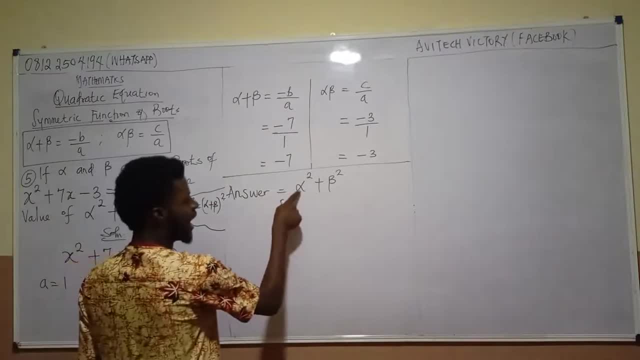 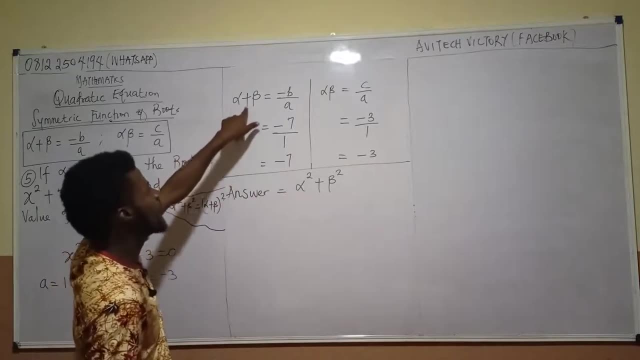 Now please look at this. This is alpha squared plus beta squared. You are squaring them individually, So you can't use alpha plus beta, because this is to the power of what and to the power of one. Now you can't use it. 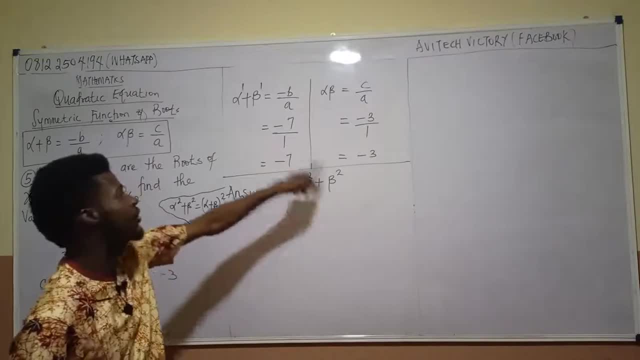 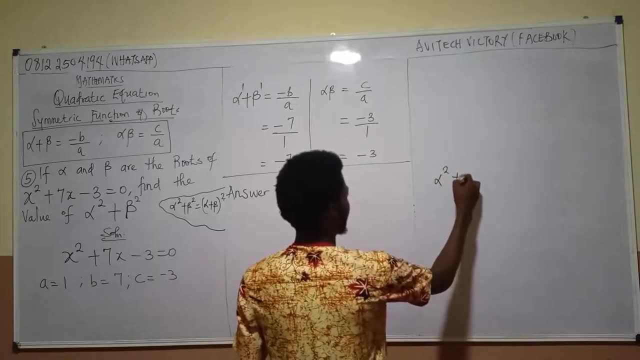 So you have to try your best to simplify this in such a way that it's going to have this and this. Now look at this. Let us see Alpha squared plus beta squared. Those of you that said it's alpha plus beta or squared. 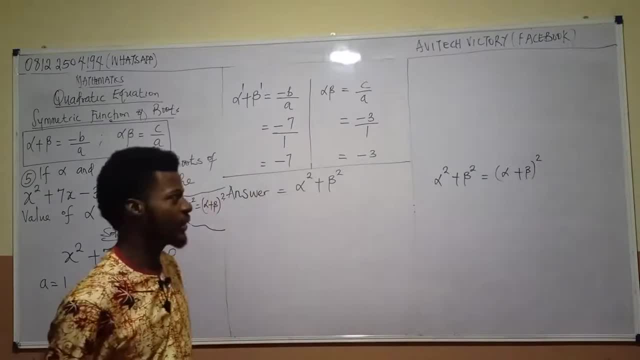 try to look at this. If you say it's alpha plus beta or squared, let us try to expand it and see what the answer will look like. Let us try to expand it Because from that point we can get our real solution. 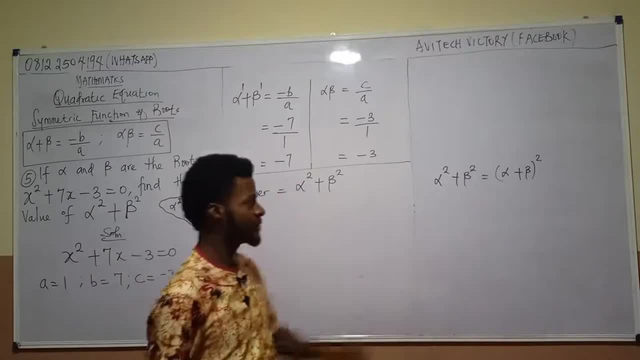 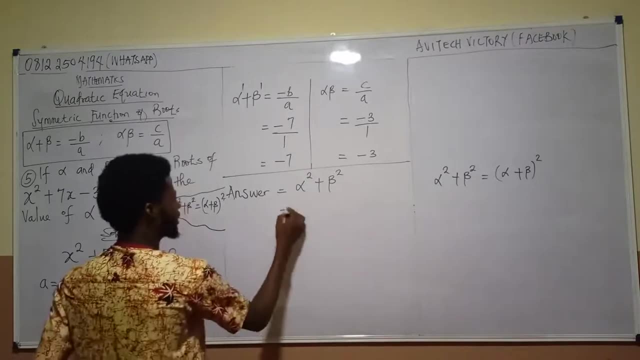 I'm not saying this is correct. I am not saying it is correct, But I'm trying to get the answer. I don't just want to write it Like I know what the answer will be. The answer of this is alpha plus beta, all squared. 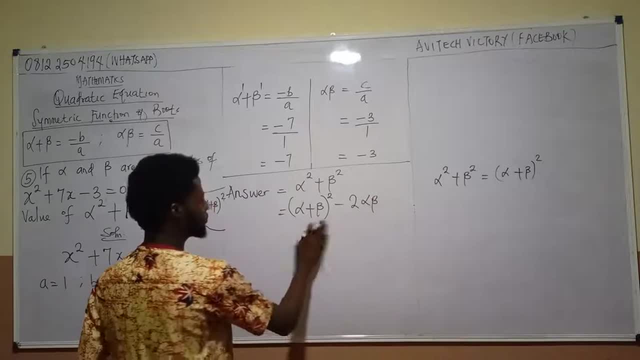 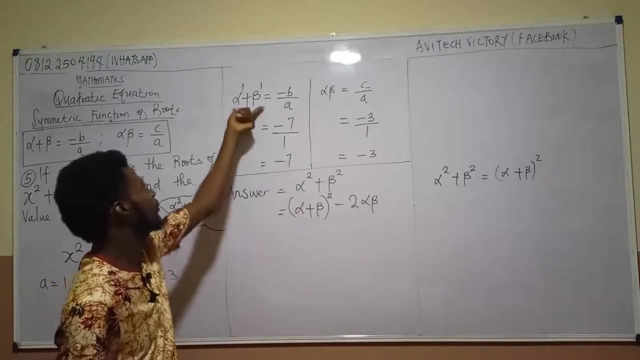 take away two alpha beta, But many people will be like, like how? But if you look at it it's kind of correct. This is alpha plus beta, which is sum of root alpha plus beta, And this is alpha beta, which is here. 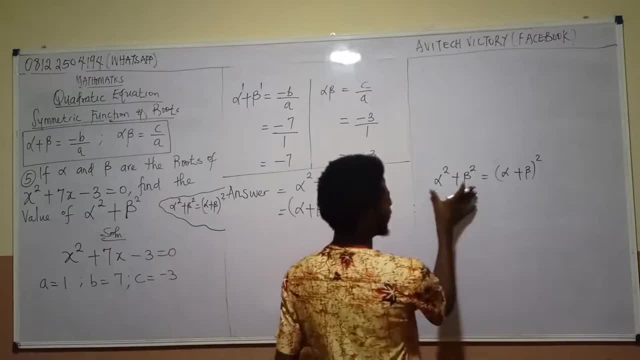 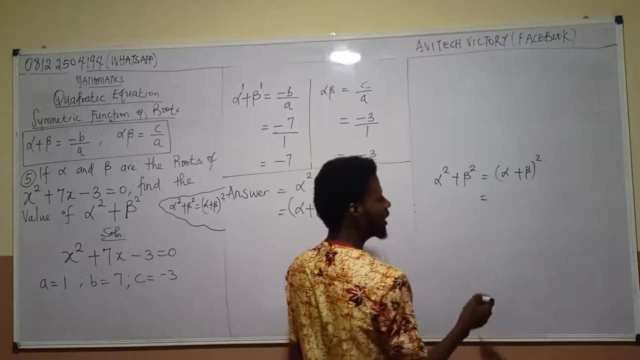 So well, let us try to do it. Look at it. So we're trying to find what expression this will be equal to. So if we say alpha plus beta squared, what does alpha plus beta squared mean? It means alpha plus beta. 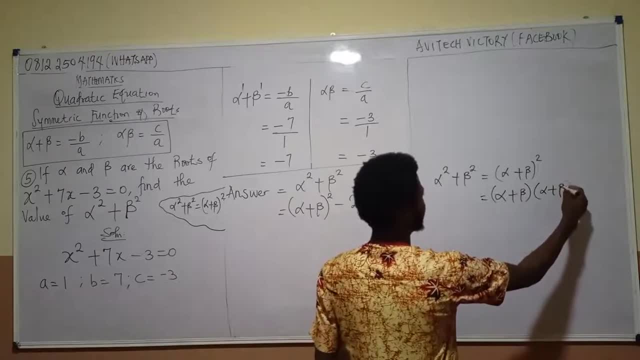 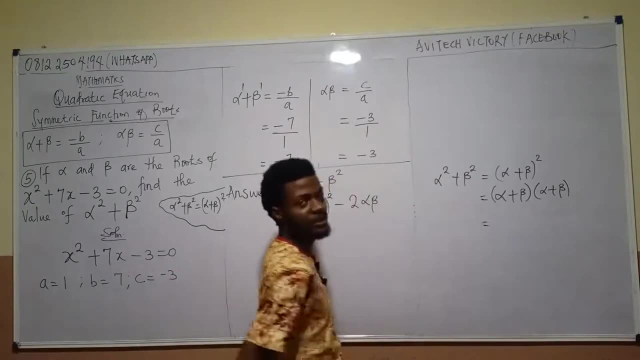 will multiply what Alpha plus what Beta. That's the meaning. So it means alpha plus beta will multiply alpha plus beta. Now the next thing is: let us expand the brackets. Alpha times, alpha, alpha squared Alpha times beta. 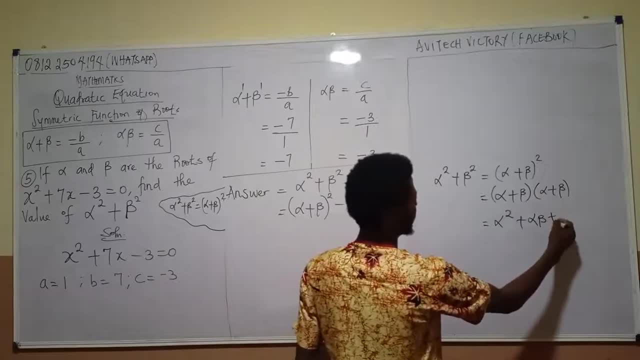 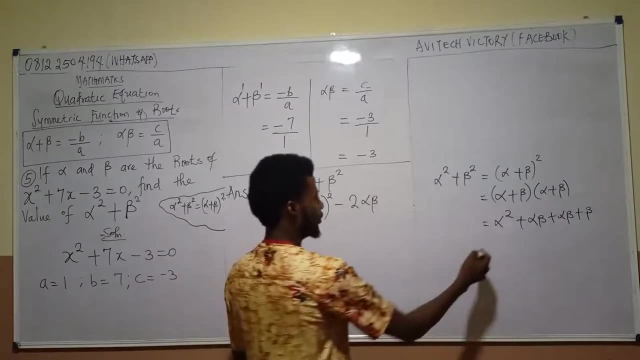 alpha beta, Beta times alpha, alpha beta. Then beta times beta. is what Beta? Now? the next thing is: this will then become: what is alpha squared? Oh sorry, This is b squared. Sorry, I'm sorry about that. 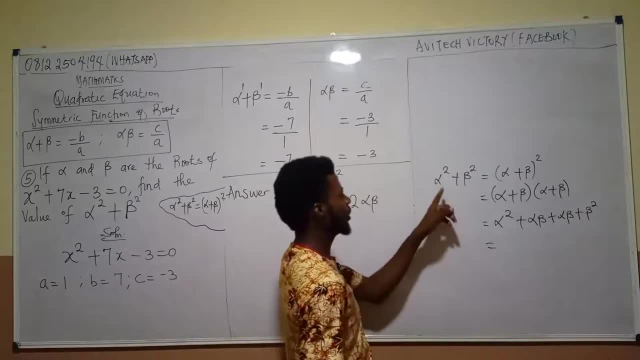 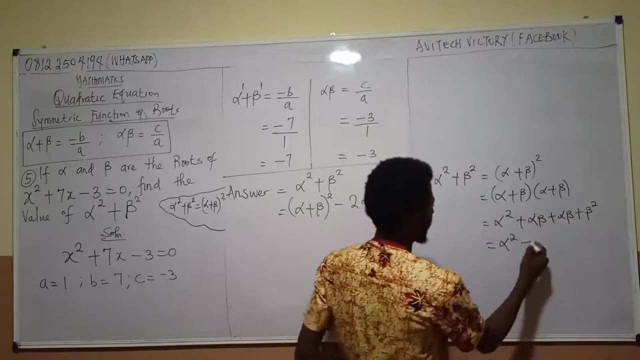 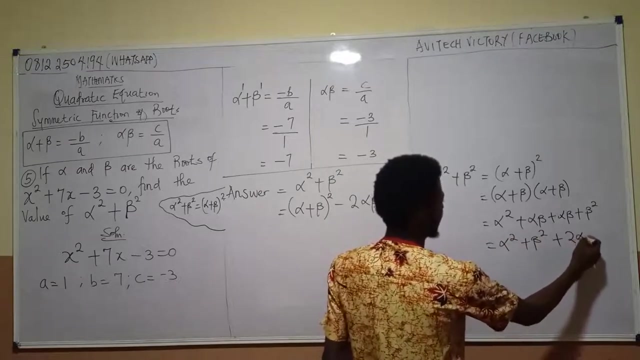 Beta times: beta is beta squared. Now, since I'm looking for alpha squared plus beta squared, let me just bring them close. This is alpha squared, Then this is plus beta squared, Then alpha beta plus alpha beta is what? 2 alpha beta. 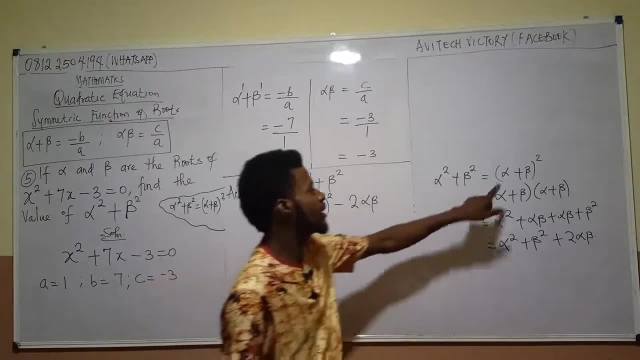 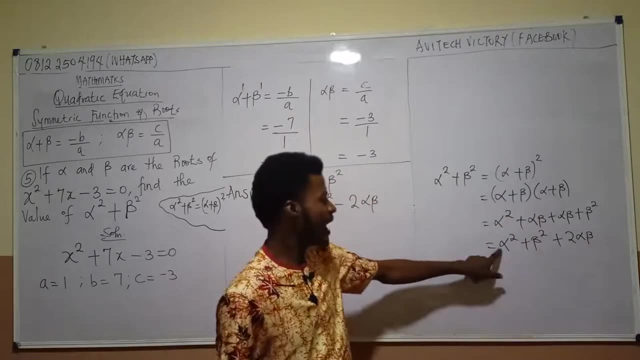 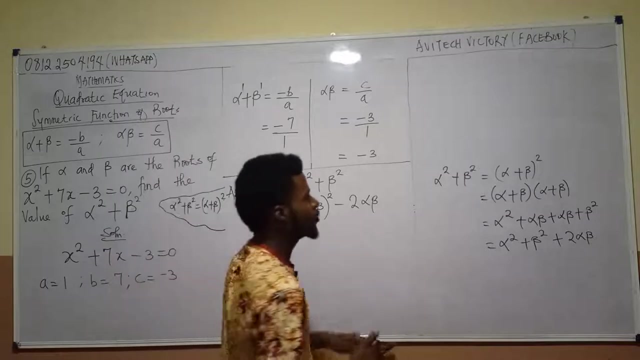 So what that means is: if you expand alpha plus beta all squared, If you expand alpha plus beta all squared, this is your answer: Alpha squared plus beta. squared plus 2 alpha beta. Now ask yourself this question. You are trying your best to make sure. 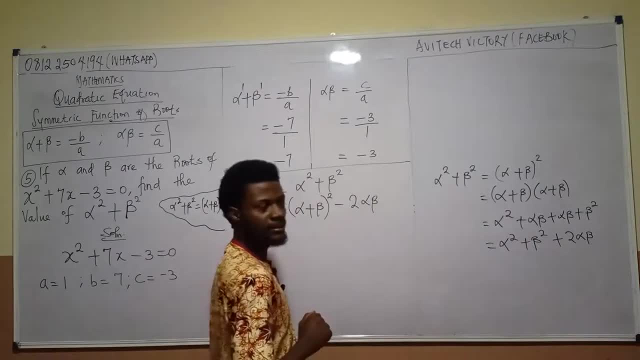 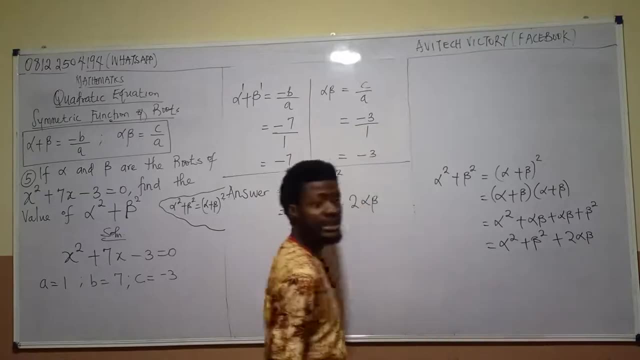 that the answer of this is the same thing as this. What is not needed here? 2 alpha beta. We do not need what 2 alpha beta It's not needed, Because if I should remove 2 alpha beta, I would then get what I'm looking for. 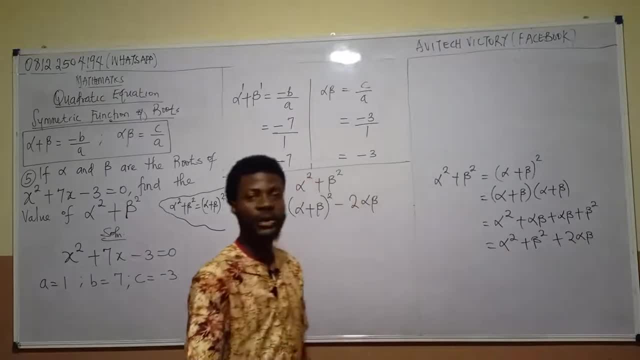 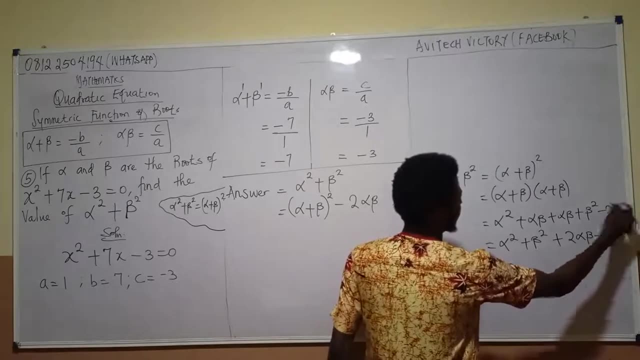 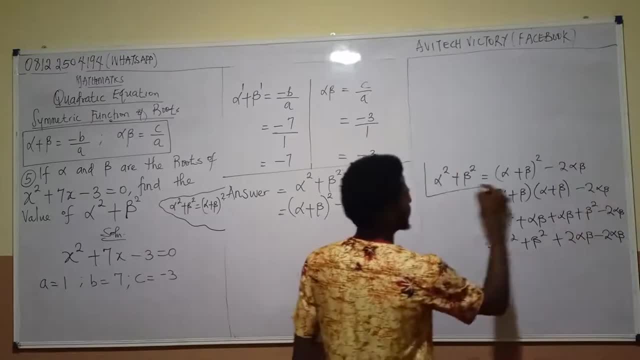 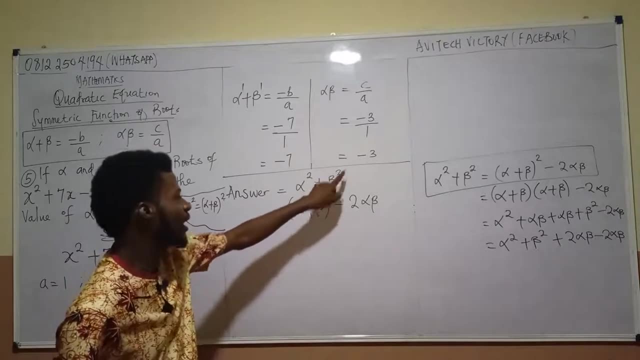 put minus 2 alpha beta here you're going to see something that this would then what Be correct? So that's why I said: alpha squared plus beta squared is equal alpha plus beta, all squared taken from 2 alpha beta. So that's why I said: 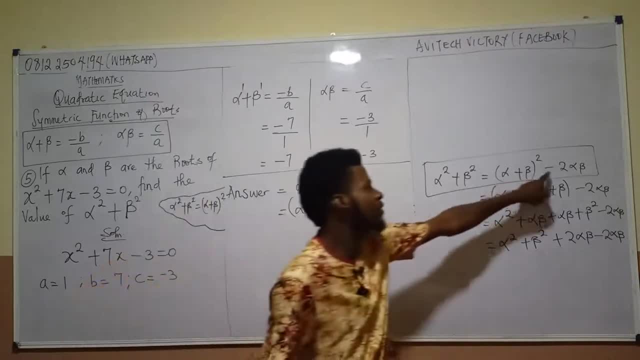 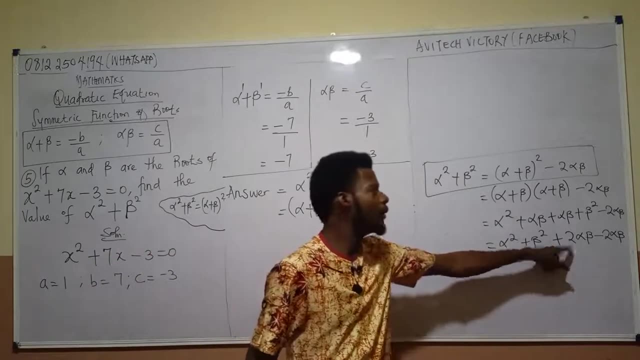 take away 2 alpha beta. That was where this minus 2 alpha beta came from, Because in the expansion of this we're going to have 2 alpha beta, But we don't need it in the expression. We don't have it in the expression. 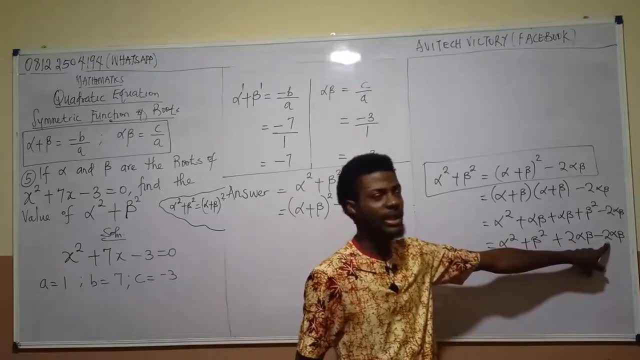 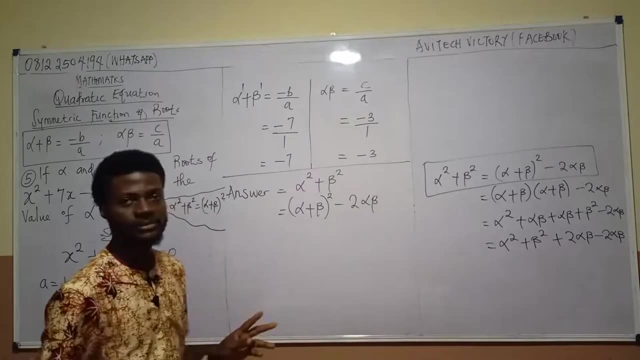 So that means I'm going to what Say minus 2 alpha beta. That's why, Remember, if you don't know the derivation, fine, Know this identity, Just know this identity. It's very important, So let us continue. 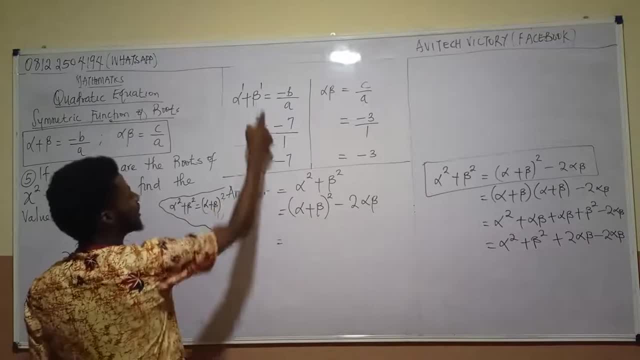 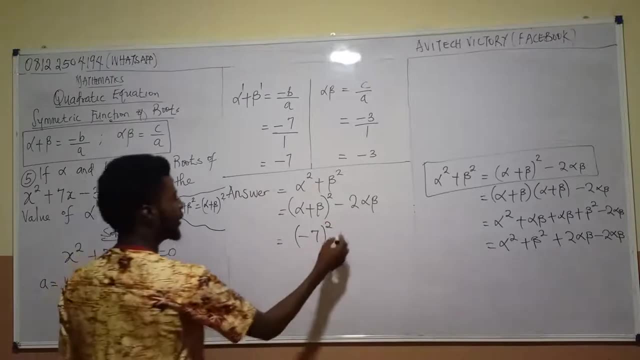 Now what is alpha plus beta? Alpha plus beta is what Minus 7.. So I'll say minus 7 all what Squared, Then minus 2 bracket, This is 2 times this. So this is minus 2 bracket. 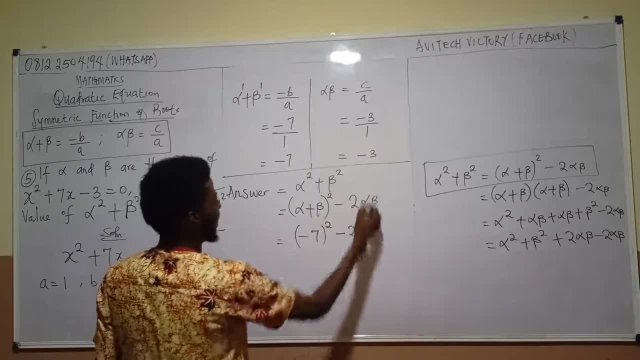 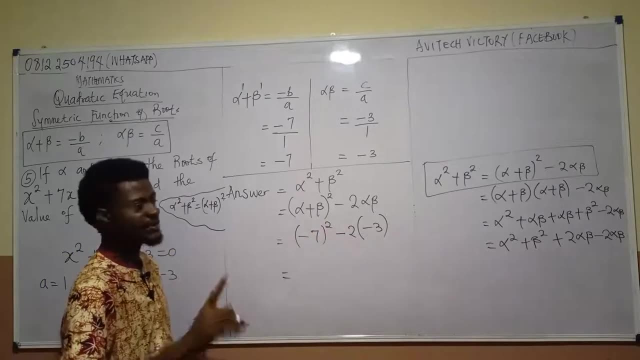 What is alpha beta? Alpha beta is minus 3.. So this will now become minus 7. squared means minus 7 times minus 7.. So that's what Minus- sorry, plus 49.. It's going to give us a plus.